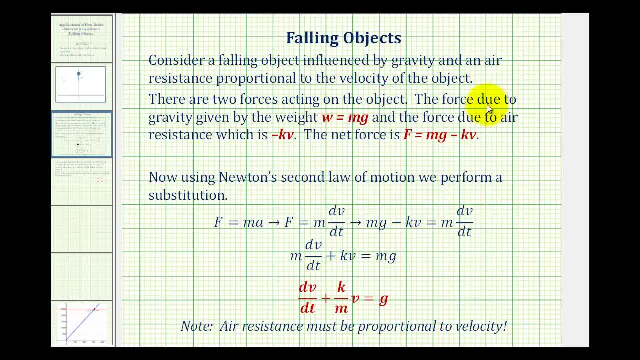 So there are two forces acting on the object: The force due to gravity given by the weight, which is going to be equal to m times g or mass times. the acceleration due to gravity And the force due to air resistance is proportional to the velocity, so it's going to be equal to negative k times v. 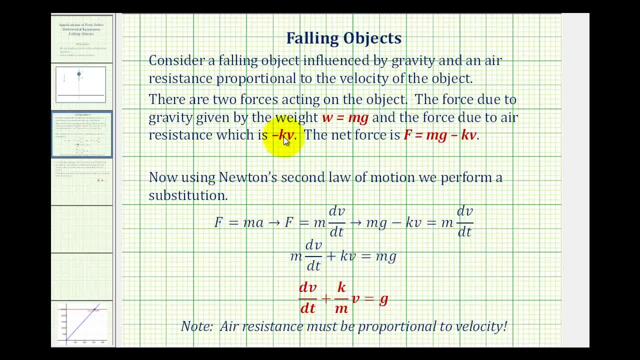 Where k is the constant of proportionality, and it's going to be negative because it's going to be in the opposite direction of the force due to gravity. So the net force, or big F, is going to be equal to m times g. 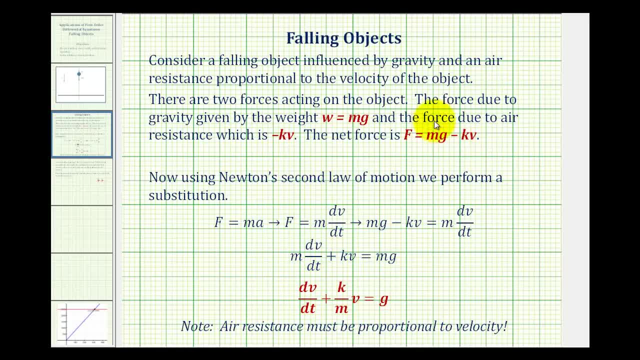 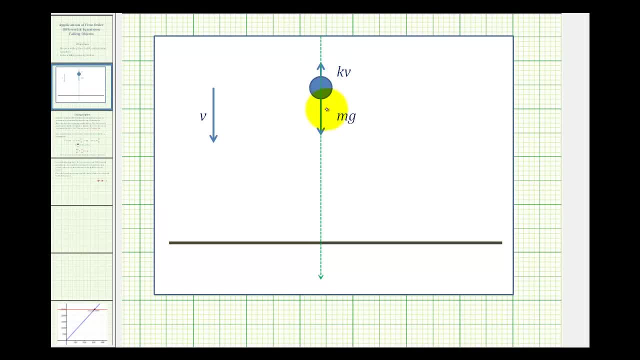 minus k times v. Let's take a look at a diagram to get a better feel for what's happening here. If this circle represents our falling object, the force downward again is going to be m times g, So in this case downward will be the positive direction. 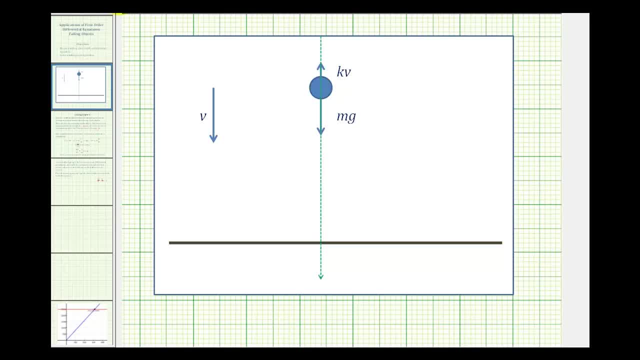 And therefore the force of the air resistance. we're going to label negative k times v, because it's going to be in the opposite direction of the force, downward, And this horizontal line here would be the ground. Now let's see how we can come up with our differential equation to model this falling object. 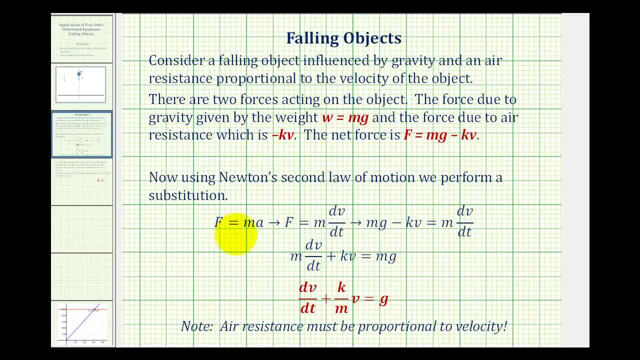 Using Newton's second law of motion, we know force is equal to mass times, acceleration, where F equals m times a. Well, the first thing we can do is replace acceleration with the v? dt, or the change in velocity with respects to time. Next, we now know that our net force, or big F, 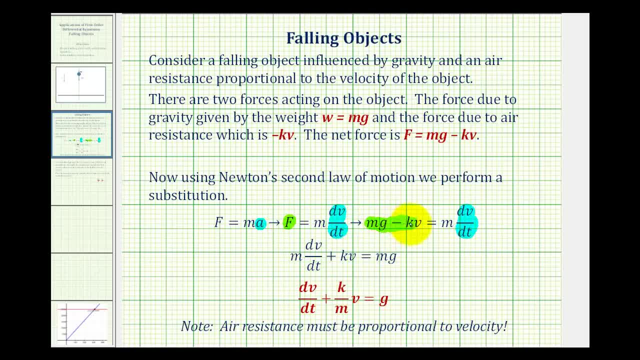 is equal to mg minus k times v. So here's a differential equation that we can use to model the falling object. but we do want to change the form of this differential equation. So the next step: we're going to add kv to both sides of the equation. 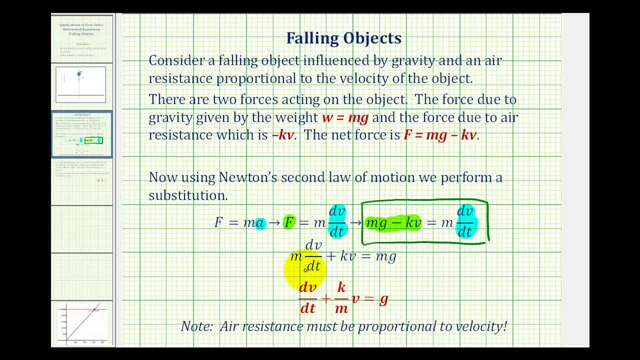 which would give us this equation here, And because this is a linear first order differential equation, we want to write this in standard form. So we'll divide both sides of the equation by m, Notice how this first term would be dv- dt. The second term would be k divided by m times v. 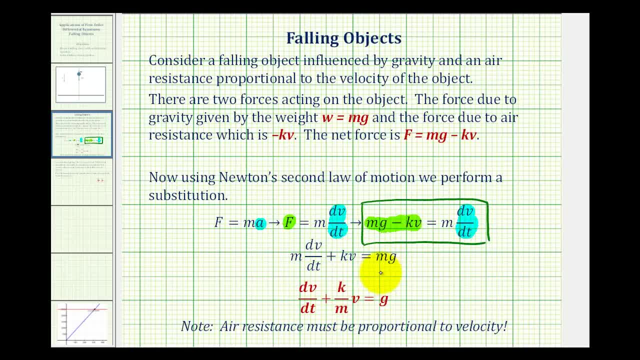 Then on the right side, the m's would simplify to one, leaving us with g. So the differential equation that we're going to use to solve our problem is dv, dt plus k, divided by m times v, equals g. It's important to recognize this only works when. 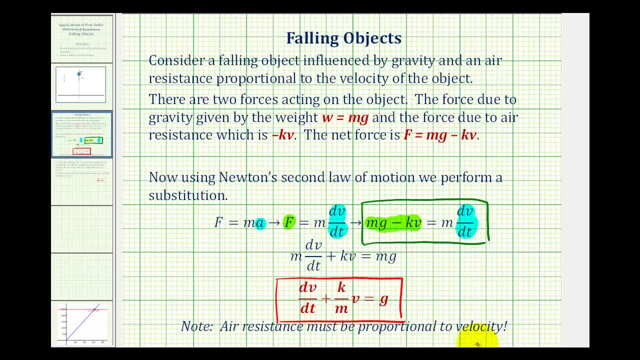 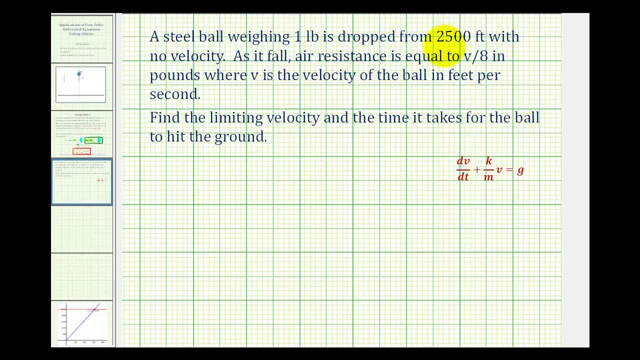 air resistance is proportional to the velocity. Now let's take a look at our example. A steel ball weighing one pound is dropped from 2,500 feet with no velocity As it falls. air resistance is equal to v divided by eight or one eighth times v in pounds, where v is the velocity of the ball in feet per second. 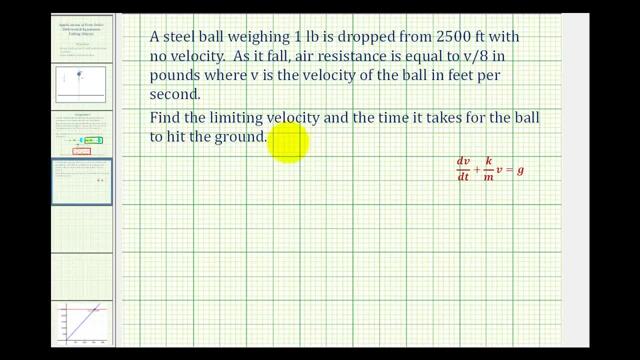 We want to find the limiting velocity and the time it takes for the ball to hit the ground. So, to set up our differential equation, we want to find k, m and g. Let's start with g, which is the acceleration due to gravity. 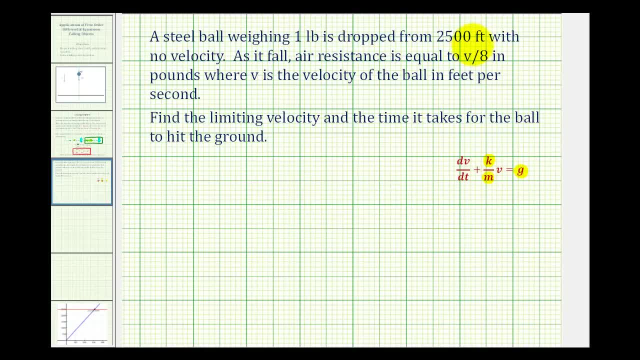 Because in this problem we're dealing with feet. the acceleration due to gravity is going to be 32 feet per second. squared, or, g equals 32.. Again, we're using a positive value here because we're assuming downward is the positive direction. 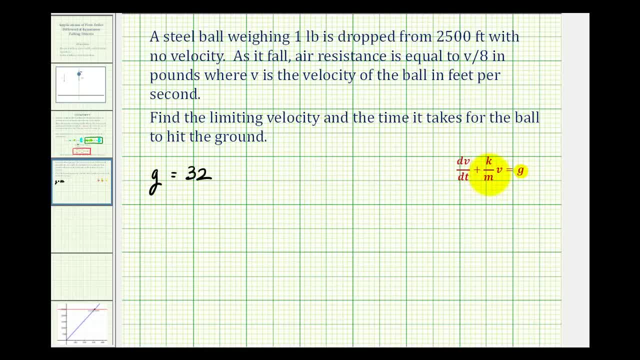 Now we need to find k and v. Let's talk about k, which relates the air resistance to the velocity. Well, we're told that the air resistance is divided by eight pounds, or one eighth times v. That means k is equal to one eighth. 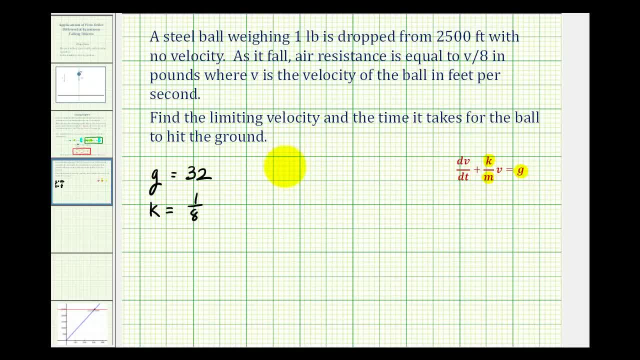 And then for the mass we need to use the equation: w equals m times g. We're told the weight is one pound, so w is one. We don't know the mass, but we know g is equal to 32.. So we have 32m. divide both sides by 32.. 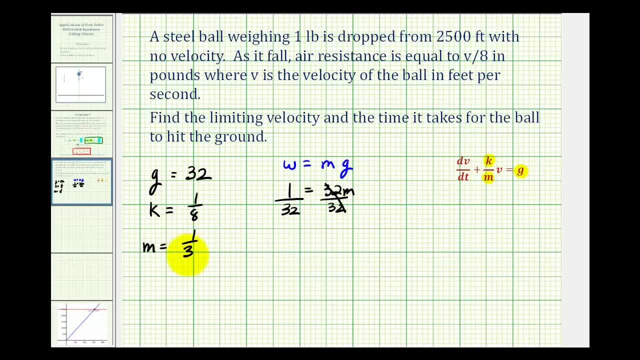 So we have g plus g plus m squared over 32.. And then we have the mass. We're told that g plus g plus m squared over 32 is equal to one over 32 slugs or just one over 32.. This gives us all the information we need to write our differential equation. 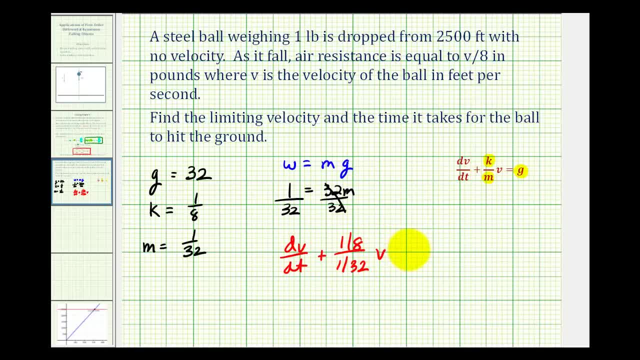 We have dv dt plus. this would be one eighth over one over 32, times v must equal positive 32.. divided by 1 over 32 is going to be 4.. So we have dv dt plus 4v equals 32.. Again. 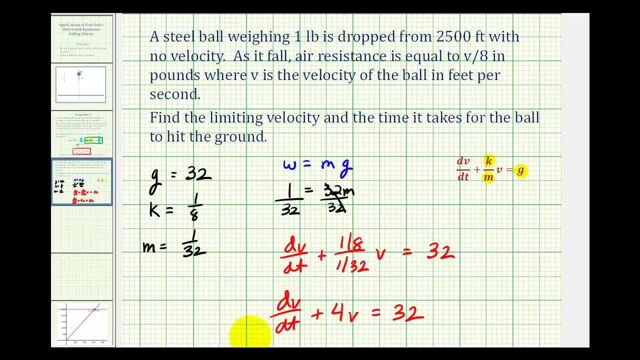 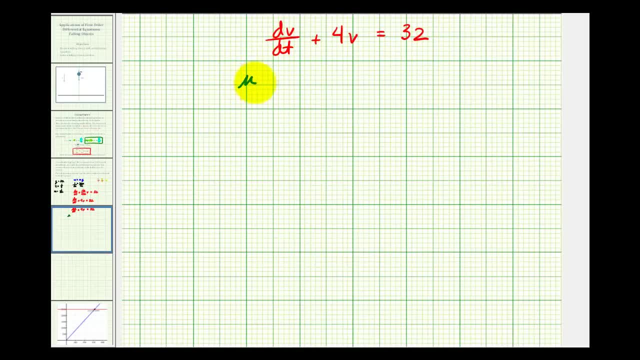 this is a linear first order differential equation, so we're going to solve this using an integrating factor. Let's go ahead and do that on the next slide. Our integrating factor, mu of t, is going to be equal to e raised to the power of the integral of the function being multiplied by v, or in this case, just the. 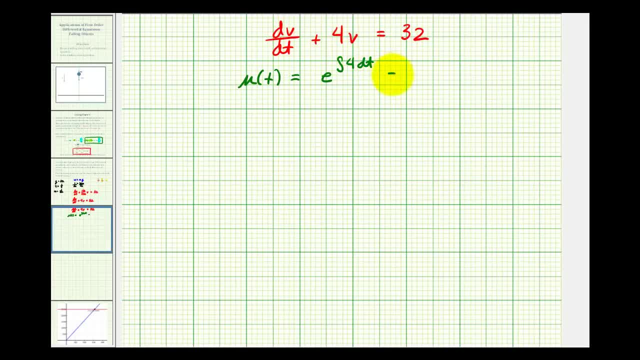 constant 4 dt. So the integrating factor here is going to be e to the power of 4t. Now we're going to multiply everything in this equation here by our integrating factor. Now, when using an integrating factor to solve this linear first order, 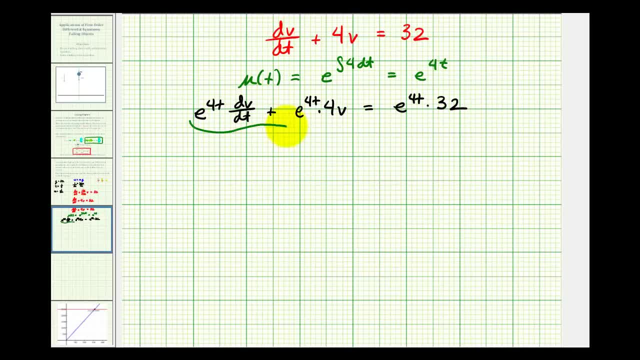 differential equation. the left side of this equation, or this side here, is always equal to the derivative of the product of the integrating factor and our function v. So if the left side is equal to this derivative, this derivative must also be equal to the right side, or 32e to the 4t. And now we can solve this by: 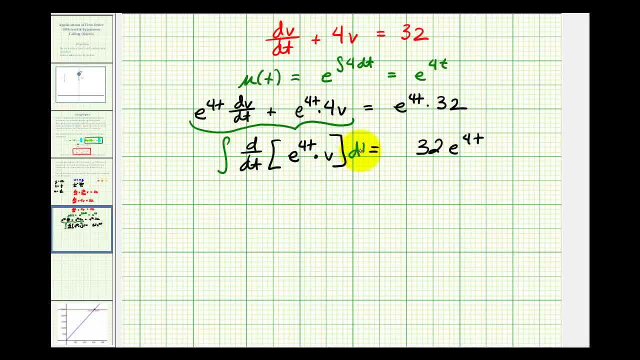 integrating both sides of the equation with respect to t. On the left side, the integral and derivative undo each other, So we're left with e to the 4t times. v must equal. here we do have to perform a u substitution where u is going to be. 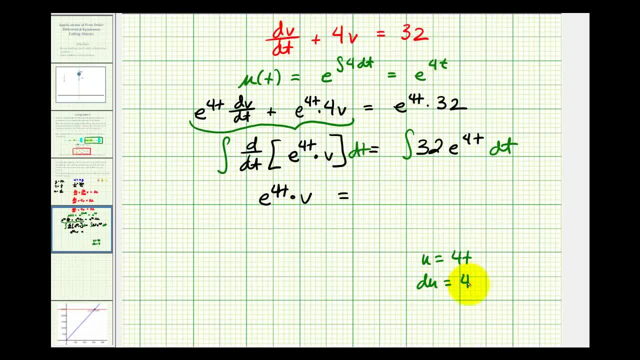 is equal to four t. so differential u is equal to four dt. dividing both sides by four. If we write this in terms of u, we'll have an extra factor of 1- 4th. so we're going to have 32 divided by four. 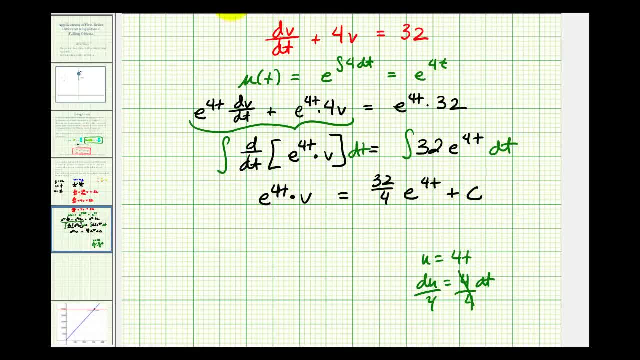 times e to the four t plus c. Now we'll solve this equation for v by dividing everything by e to the four t. So this simplifies to v or v of t. this simplifies to one, and 32 divided by four is eight. 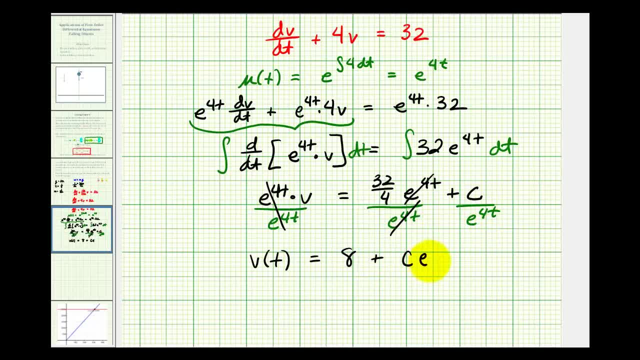 so we have eight plus. we'll write this as c times e to the negative four t power. Now we need to find our constant c. To do this, we know that v of zero is equal to zero. the initial velocity is equal to zero. 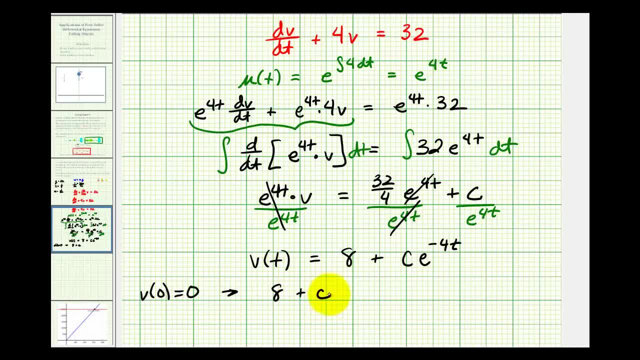 so that means that eight plus c times this would be e to the zero, or one must equal zero. therefore c is equal to zero and c is equal to negative eight. so our velocity function is: v of t equals eight minus eight times e to the negative four t. 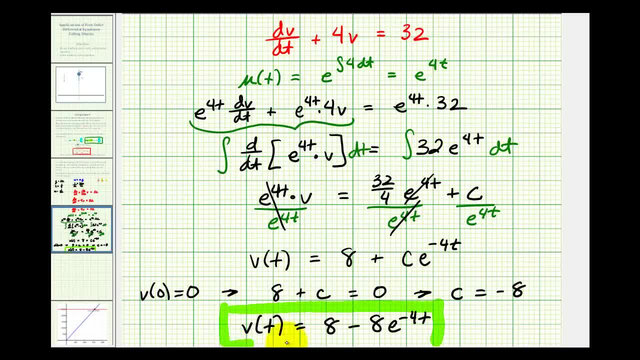 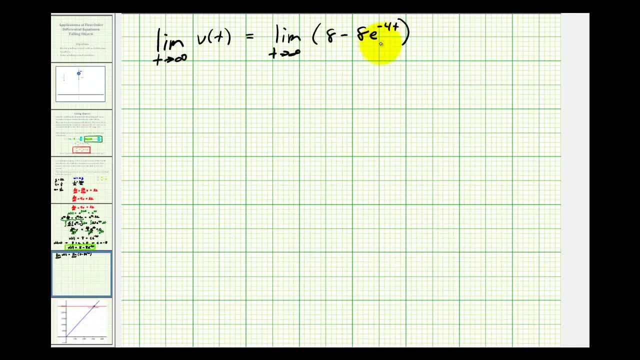 So to find our limiting velocity, we need to find the limit of this function as t approaches infinity. Let's go ahead and do that on the next slide. To do this, it might be helpful to rewrite this second term as a fraction, So we would have eight minus eight. 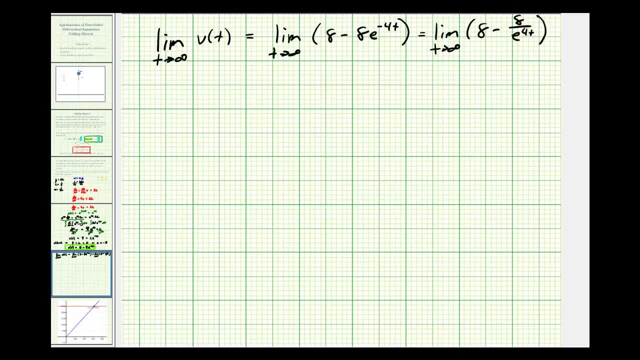 all over e to the power of four t. In this form we can see, the second term here is going to approach zero, because the denominator is increasing without bound as t approaches infinity. Therefore, this limit is just equal to eight, which means our limiting velocity. 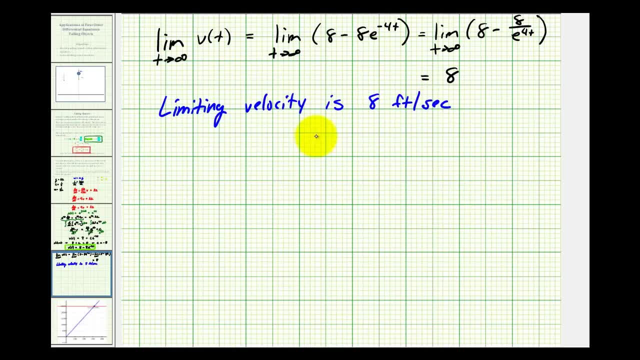 is equal to eight feet per second. That's the fastest this object will fall until it hits the ground Due to the air resistance. Now for the next part. we're asked to determine when the object is going to hit the ground. To do that, we want to find the position function. 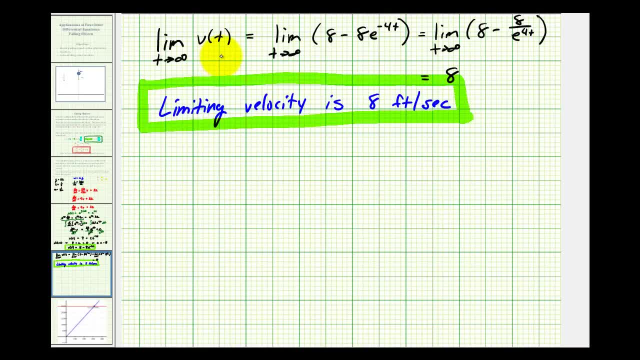 Remember, the velocity function or v of t is the derivative of the position function, which means if we integrate the velocity function with respects to t, we will be able to find the position function. So we'll have s of t equals the integral of eight. 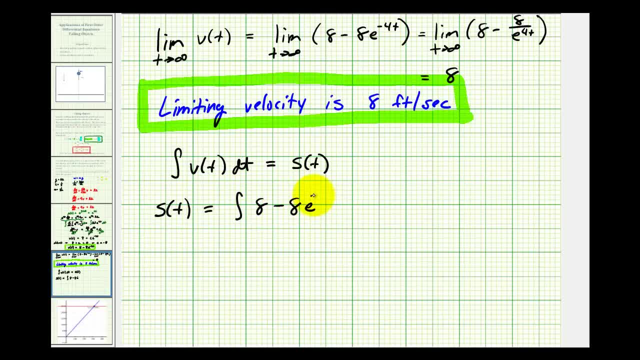 minus eight times e raised to the power of negative four t. Notice again, integrate the second term. we have to perform a u substitution where u is going to be equal to negative four t, So differential u is going to be negative four dt. 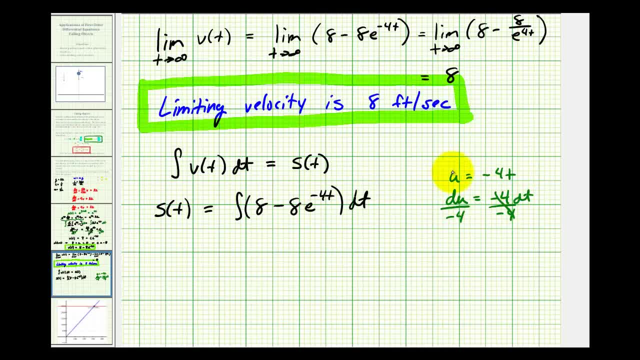 Divide both sides by negative four. So, performing the substitution, we'll have an extra factor of negative 1, 4th. So s of t is going to be equal to t minus eight times negative 1, 4th. e to the negative four, t plus c. 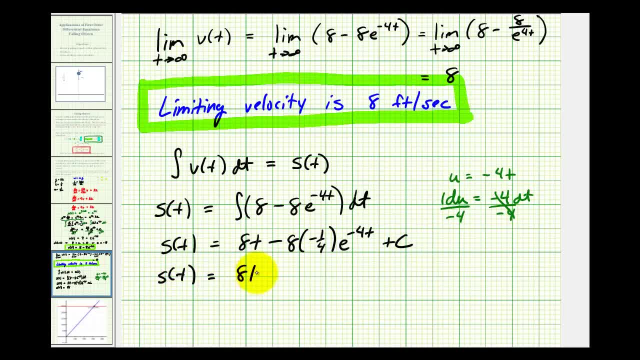 So simplifying. here we'll have s of t equals eight t. it's going to be plus two times e to the negative, four, t plus c. Now, before we find the constant of integration, let's go back to our diagram just for a moment. 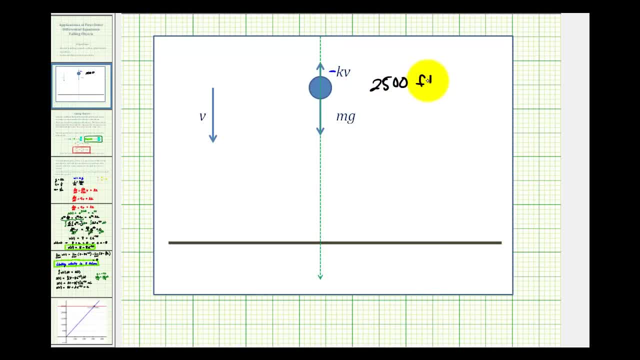 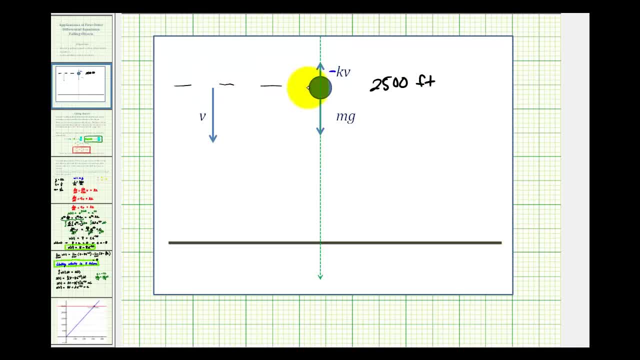 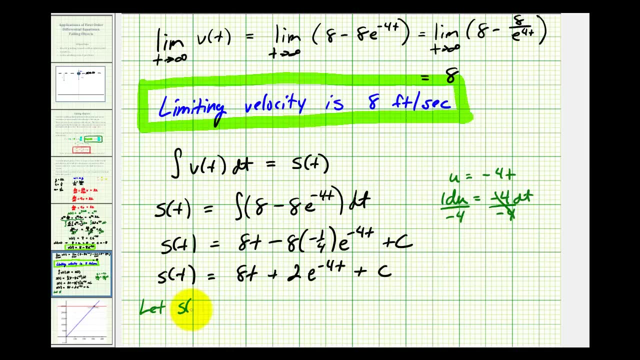 we're actually going to let this height here be zero and let the ground be 2,500 feet, So the object starts here and then, when it hits the ground, it will travel 2,500 feet. So we'll let s of zero. 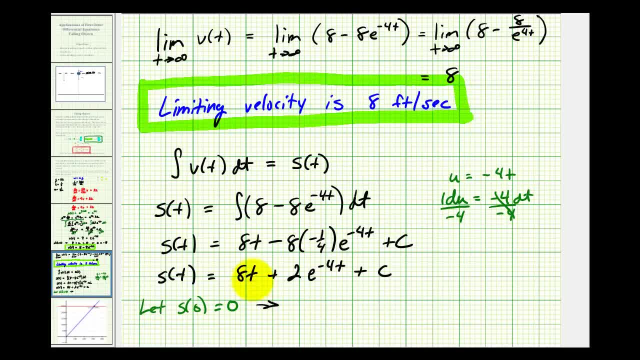 equals zero. So this would give us eight times zero, that's zero plus two times e to the zero, which is one plus c equals zero. So we know c must equal negative two. So our position function s of t is equal to eight t. 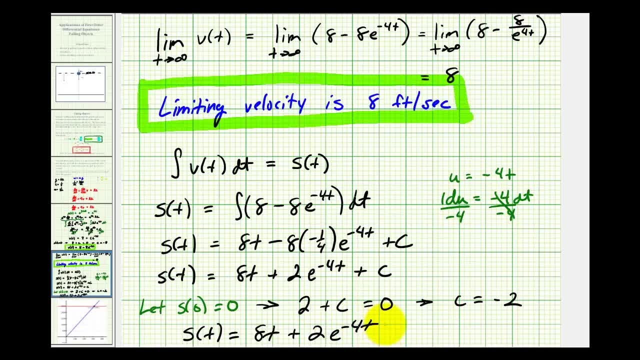 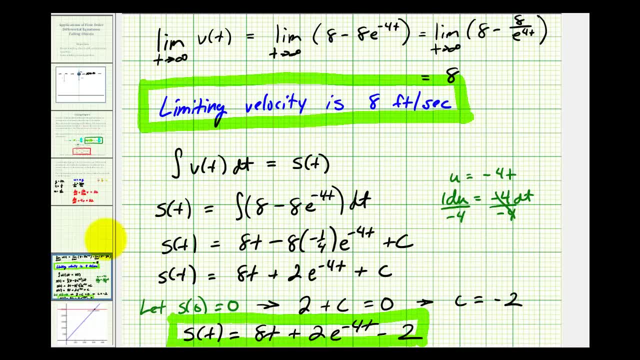 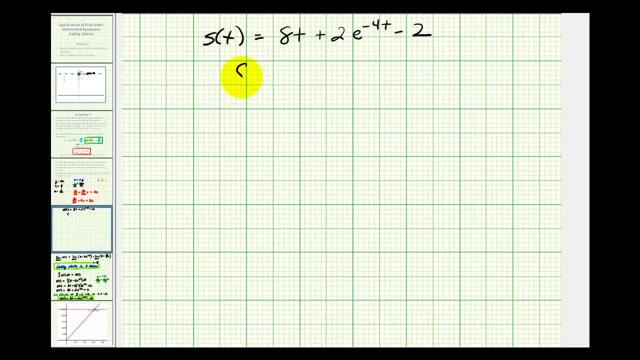 plus two times e to the negative 4t minus two. So to determine how long it's going to take for this object to hit the ground, We're going to set our position function equal to 2,500, and then solve for t. So we want to solve the equation eight t. 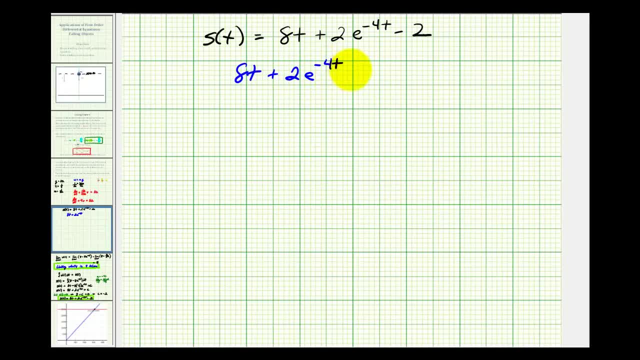 plus two times e to the n, e to the negative, four t minus two equals 2,500.. Now, solving this equation would not be easy. We would actually take trial and error by hand. So what we're going to do is solve this graphically. 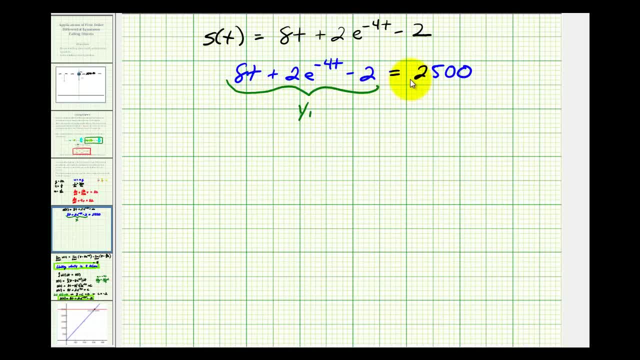 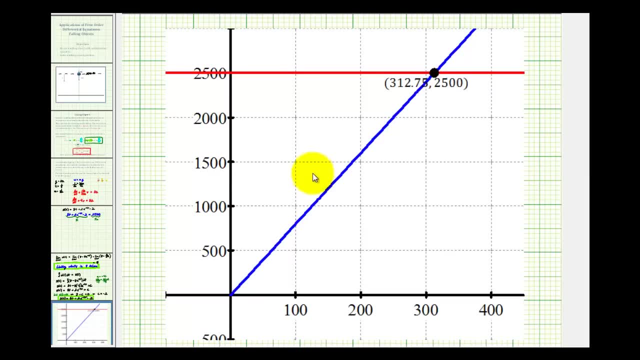 We'll graph the left side of the equation, as let's say y one, and we'll graph the right side, as let's say y two. So if we graph this, the blue graph would be the graph of the left side of the equation, or y one. 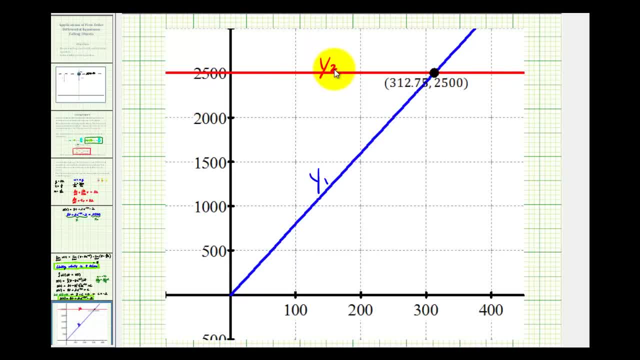 and the graph of the right side of the constant would be the red graph or y two. So this point of intersection represents our solution, because we're looking for a time that's going to be the x coordinate, So it's going to take approximately 312.75 seconds.